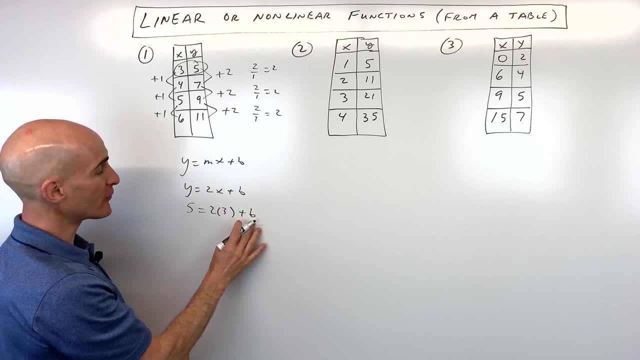 So when y is 5, x is 3, we can solve for b. So we have: 5 is equal to 6 plus b. So track 6 from both sides and you can see that b is equal to negative 1.. You just put the negative 1 back into the equation and you've got it. 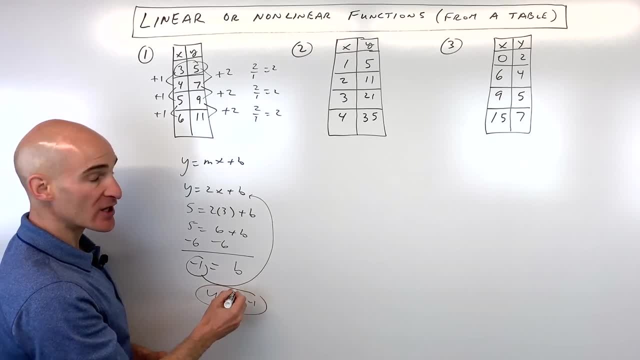 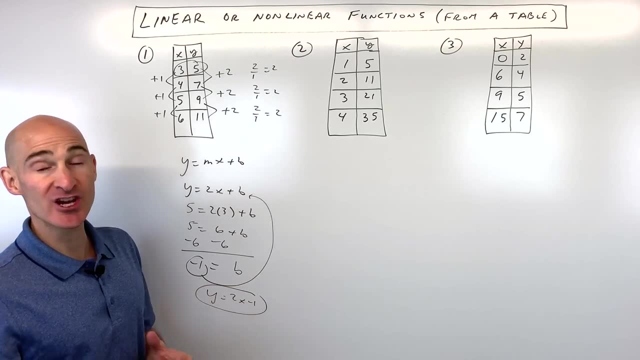 So it's: y equals 2x Minus 1.. Of course, if you want to check your work, you can always pick another coordinate. Say, for example, if x is 6, 2 times 6 is 12, minus 1 is 11.. Okay, it checks out, right. 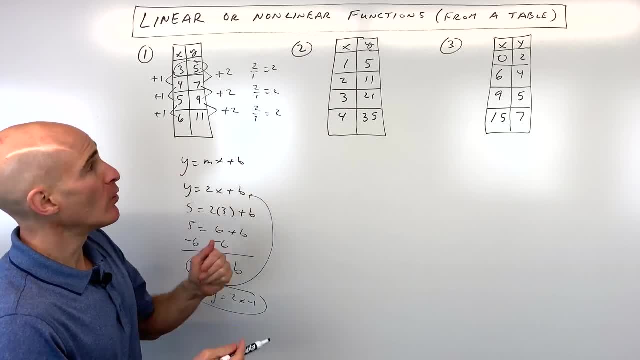 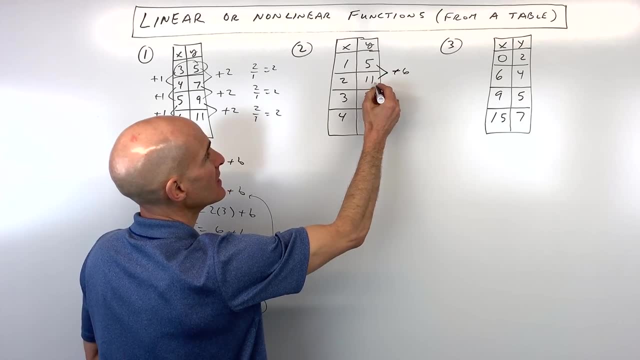 Okay, let's go to number 2 now. Is this one linear or nonlinear? Well, let's take a look at the change in y over the change in x. So when we look at how the y's are changing, it looks like they're going up by 6.. Here it's going up by 10.. 21 to 35, it's going up by 14.. 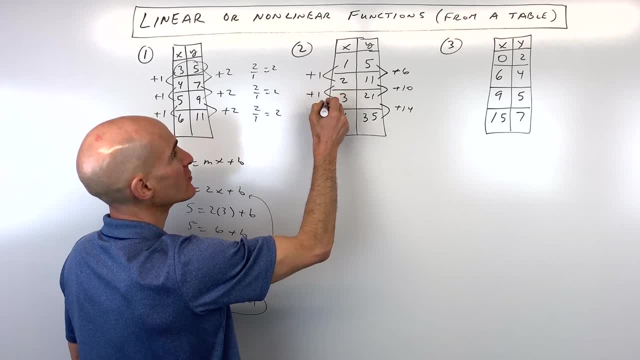 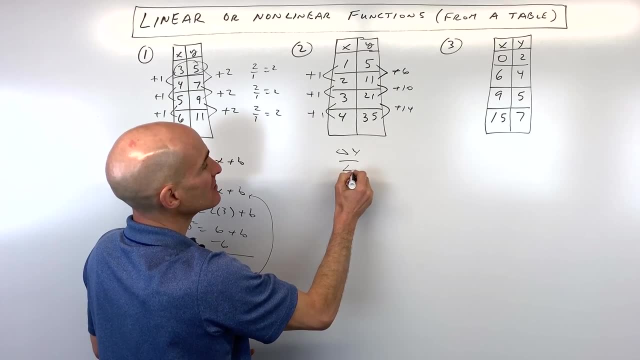 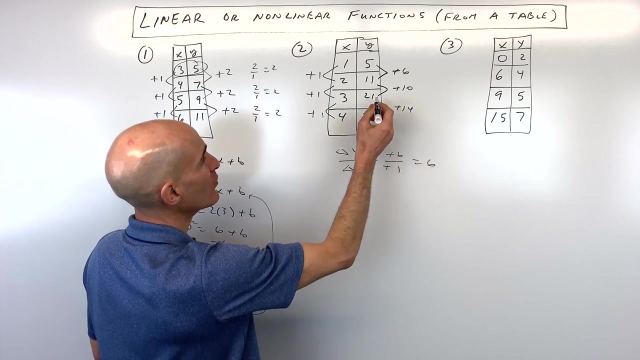 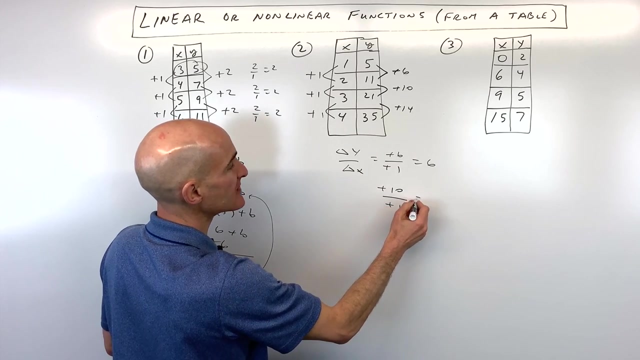 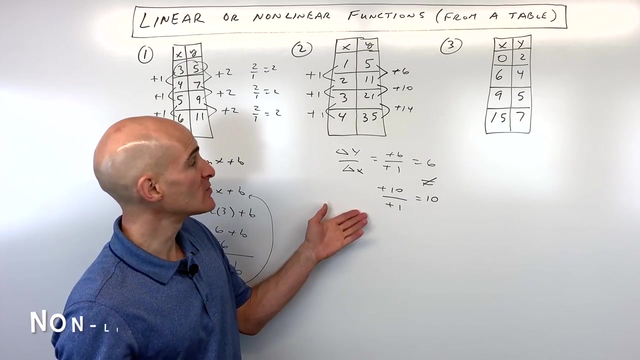 When we look at the change in x, it looks like it's going up by 1.. 2 to 3, it's going up by 10.. 3 to 4, it's going up by 1.. But when we look at the change in y over the change in x, right, So here it's going up by 6.. When the x's are going up by 1, that's the slope of 6.. But when we look at over these two points, here it's going up by 10 in the y direction. When the x's are going up by 1, that's the slope of 10.. You can see, 6 does not equal 10, which means it's not going up at that steady, constant rate, which means that this one is going to be nonlinear. 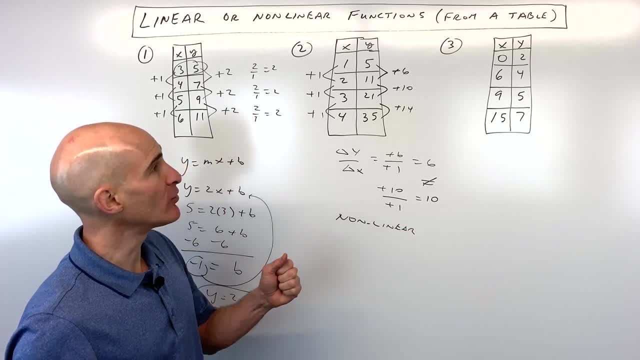 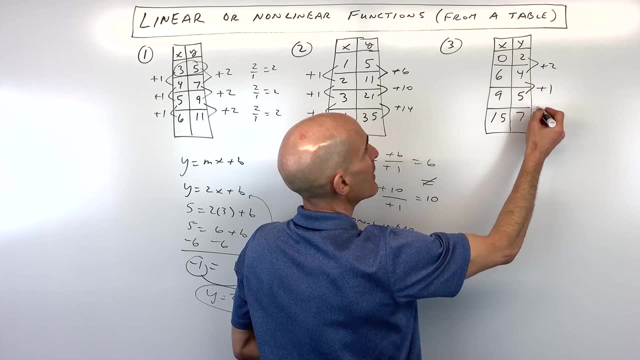 Okay, meaning not a straight line. Okay, last example, number 3.. See if you can do this one. Let's look at the change in y. It looks like the y's are going up by 2.. Then they're going up by 1 here. Then they're going up by 2 here. 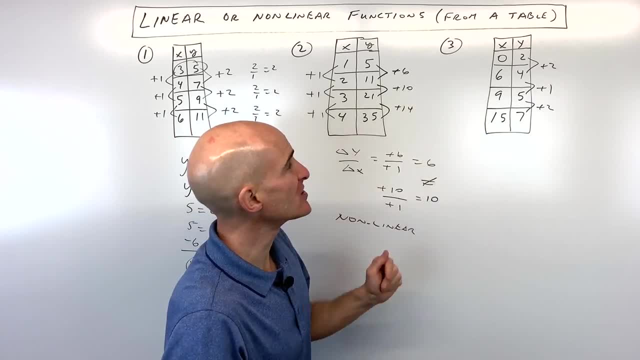 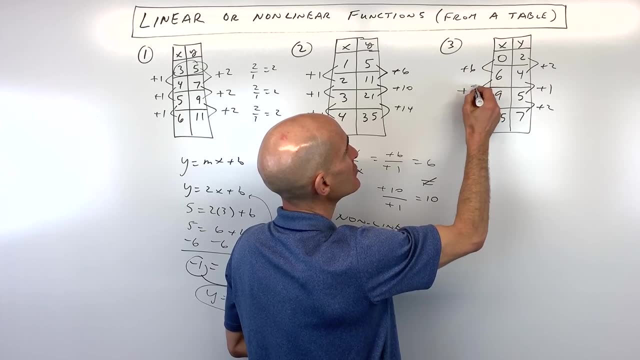 Now it's okay that they're not going up at the same for each one. What we're interested in is the change in y over the change in x. Is that slope the same? So here it's going up by 6.. Here it's going up by 3.. Here it's going up by 6.. 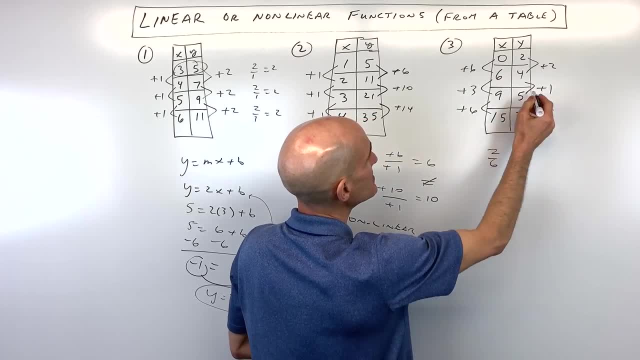 If we take the change in y over the change in x, we're getting 2 to 6.. 1- 3rd and 2- 6th. But you can see that 2- 6th reduces to 1- 3rd. 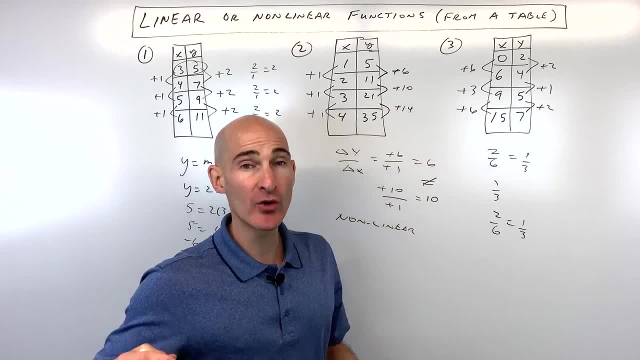 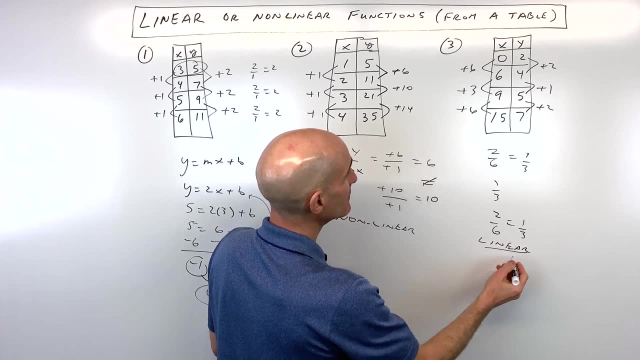 Okay, so we have 1 3rd equals 1, 3rd equals 1, 3rd. So this is actually going up at a constant rate with a slope of 1- 3rd. So this is linear. If we want to write the equation of this linear function, this line, we're going to take our y equals mx plus b. 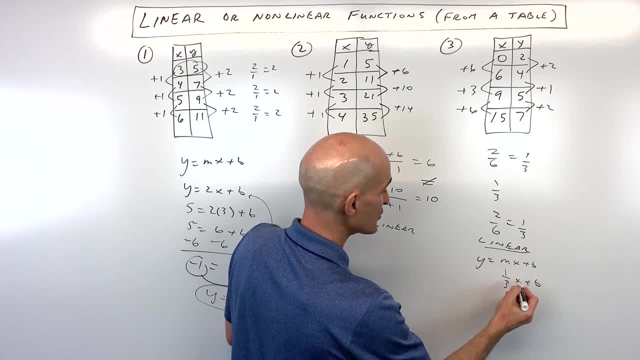 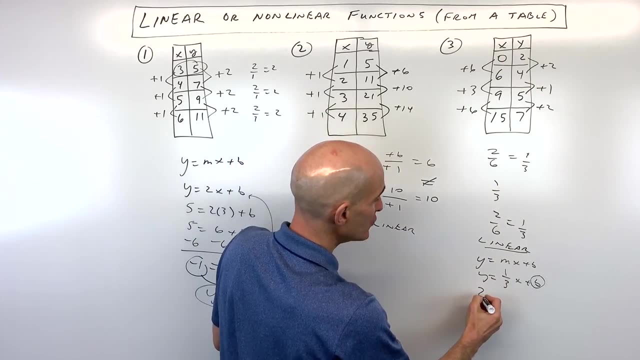 We know our slope is 1- 3rd, but we have to solve for that b value, that y intercept. Okay, so let's pick one. So we have two points here: 0 comma 2.. So if you put 2 in for y and 1 in- sorry, 0 in for x, we can solve for b. 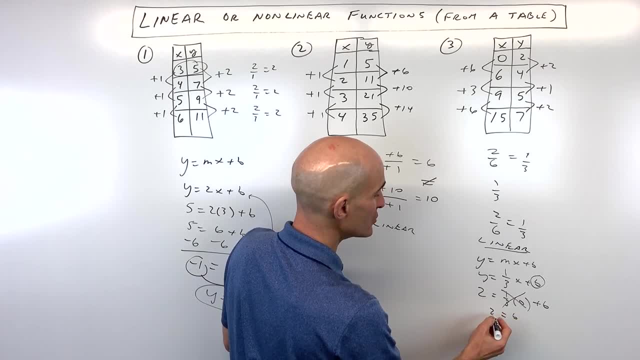 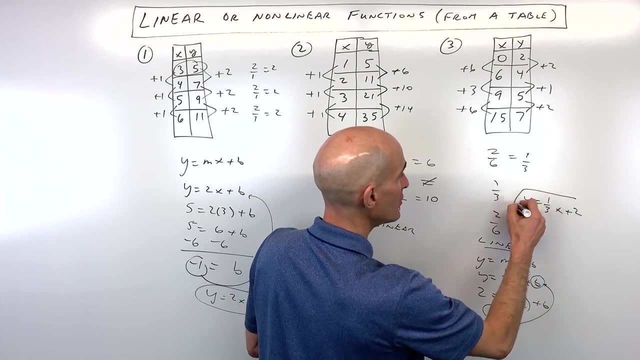 1, 3rd times 0 is 0. So you can see b is equal to 2.. So if we put the 2 back in to our equation, we've got it. So y equals 1, 3rd x plus 2, and that's the equation of our line. 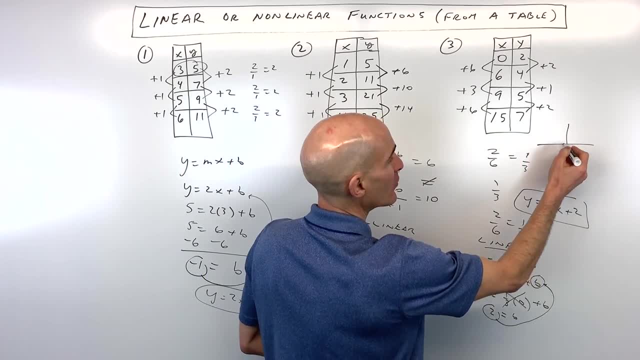 Now when x is equal to 0, you know, when you think about it you're not going left to right, You're just going up and down along that y axis. So really we knew that the y intercept was 2 in this particular example.